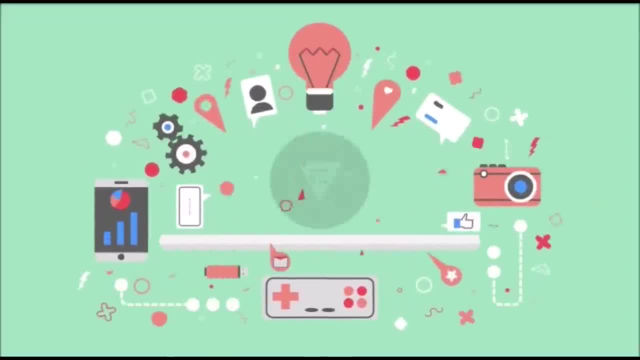 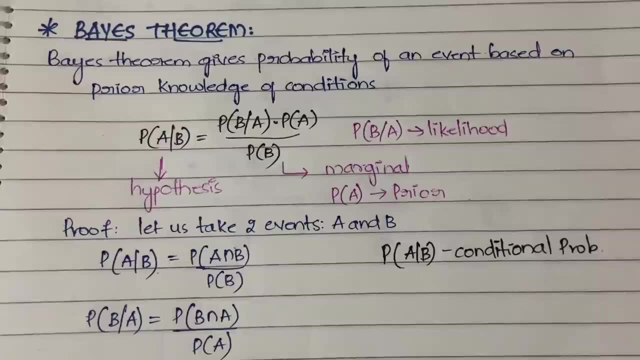 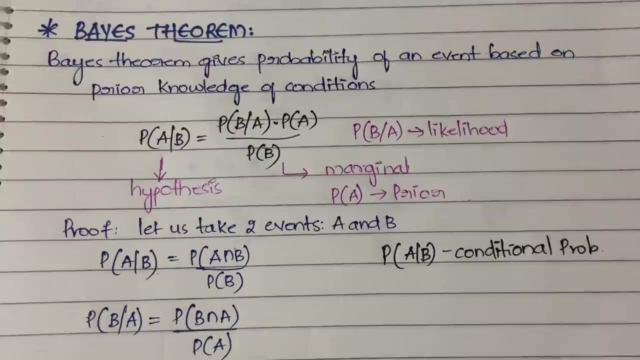 Hello everyone, welcome back to my YouTube channel, Trouble Free. In today's video I'm going to explain you about the Bayes Theorem in the subject of machine learning. So actually we have this Bayes Theorem not only in machine learning, we have it in data warehouse and data mining as well. 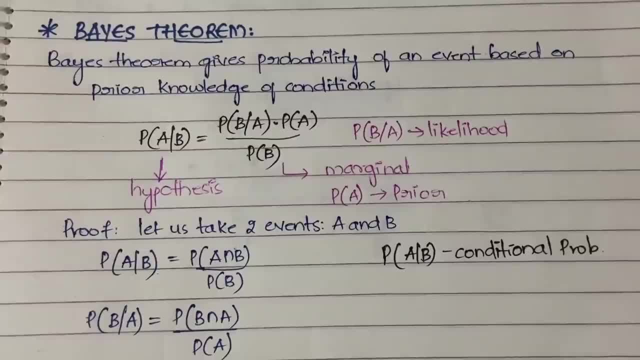 So it's very important that you understand this Bayes Theorem, Even in probability and statistics also, you'll have this, And the prerequisite for this Bayes Theorem is the conditional probability. So even if you don't know about conditional probability, that's okay. 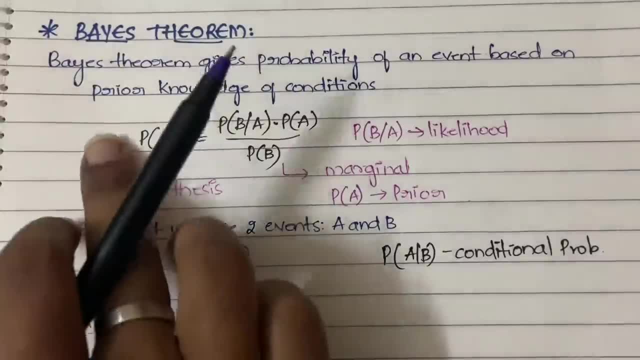 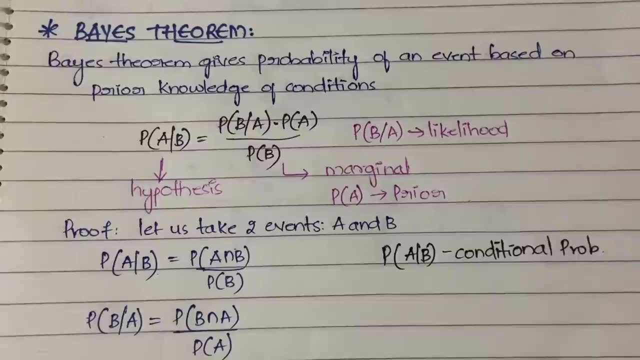 That's fine, It works. So simply, this formula stands for conditional probability, Okay, Yeah. So before starting the video, let me tell you something. If you're having your exams scheduled nearby, just let me know the date of your exam, along with your college name in the comment section, so that I can make videos by your exam date and also according to your college syllabus. 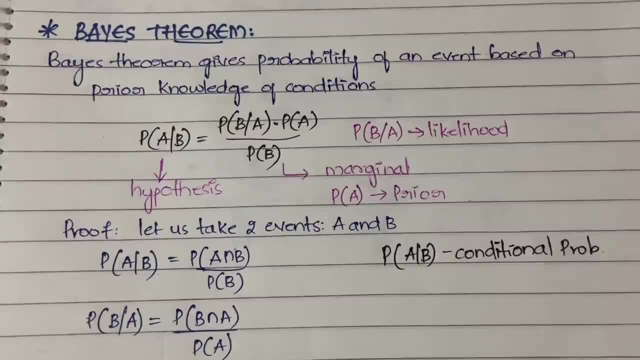 And also let me know what is the next playlist that you people want me to make videos on. Okay, So let's get started without any further delay. So first, what do you mean by Bayes Theorem? The Bayes Theorem will give the probability of an event based on the prior knowledge of conditions. 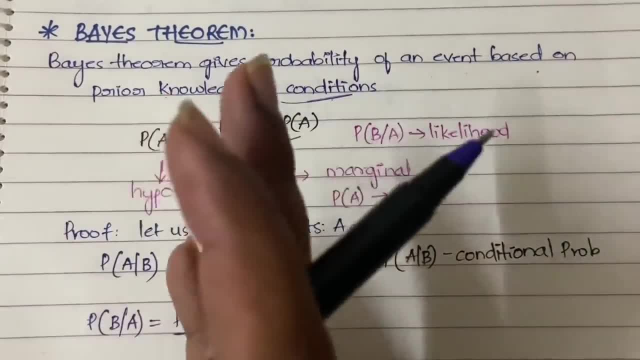 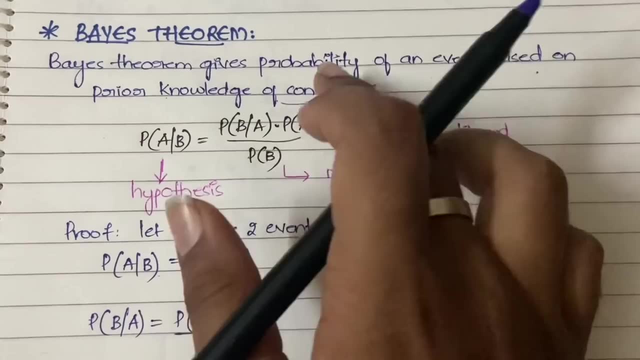 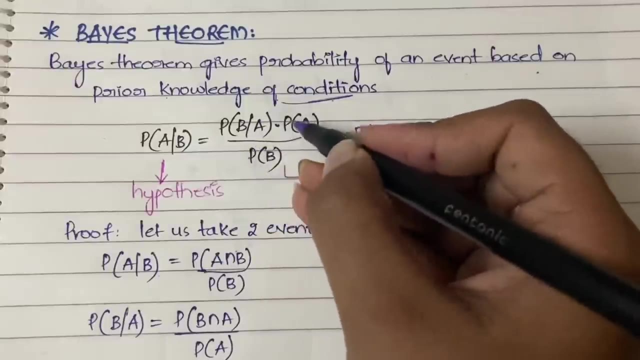 So, based on the previous knowledge, whatever the machine is having, based on those conditions, based on that knowledge, it will give the probability of an event. Okay, So simply, P of A by B is equal to P of B by A. into P of A by B. 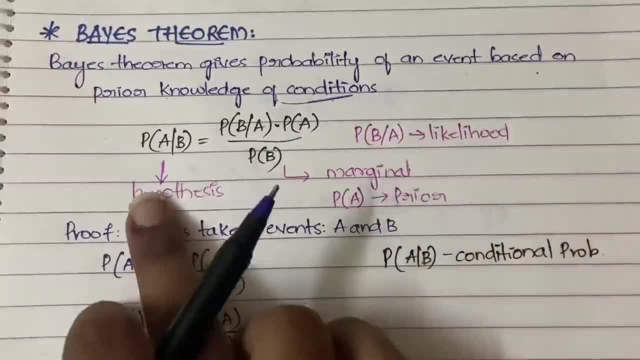 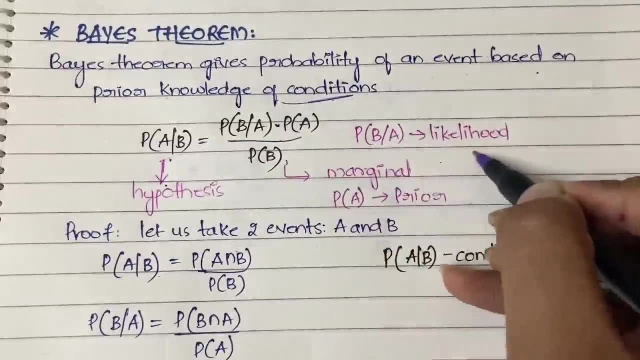 P of B. Okay, In this we actually have some terms: P of A by B is called as the hypothesis and P of B by A is called as the likelihood, and this P of B is called as a marginal and P of A is called as a prior. 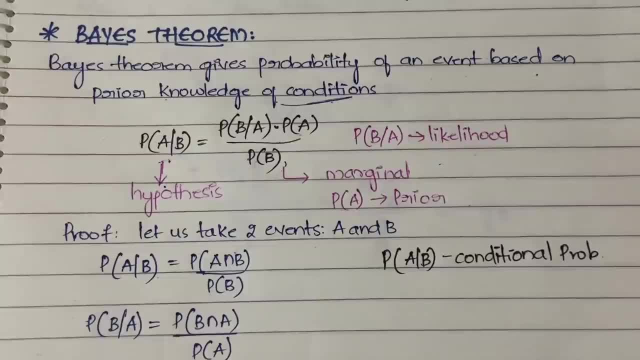 So what they are, I'll tell you in detail. Don't worry, By the end of the video you'll understand everything. Now don't worry for anything. Okay, So it is P of A by B, Right? So how do you read that? 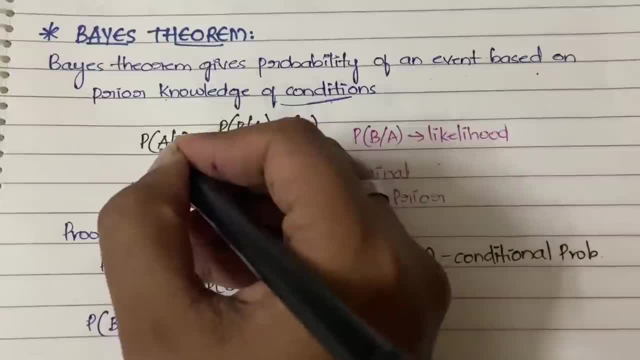 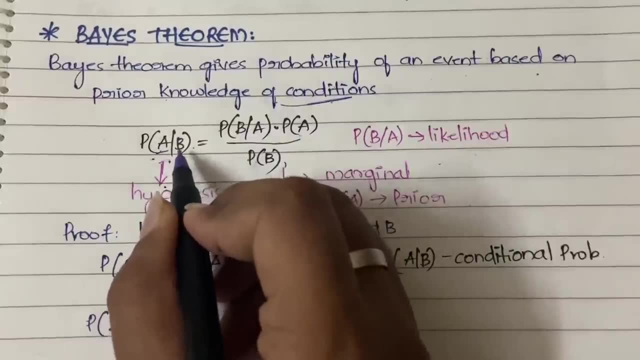 How do you read? P of A by B: Probability of A. You're finding probability of A by B. You're finding probability of A given that probability of B or given that B has already occurred. Right, So you know the probability of B. You're finding out the probability of A now. 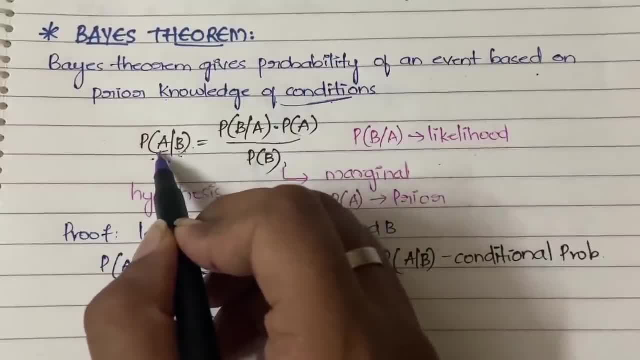 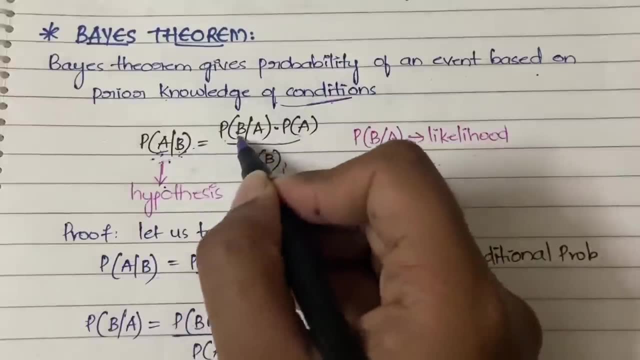 Okay. So P of A by B is finding the probability of A, given that B has already occurred. Okay, Here, finding the probability of B, given that A has already occurred. Okay, Done. This is how you need to read A by B as. 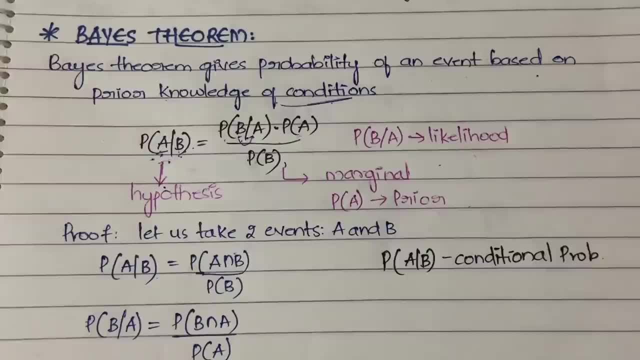 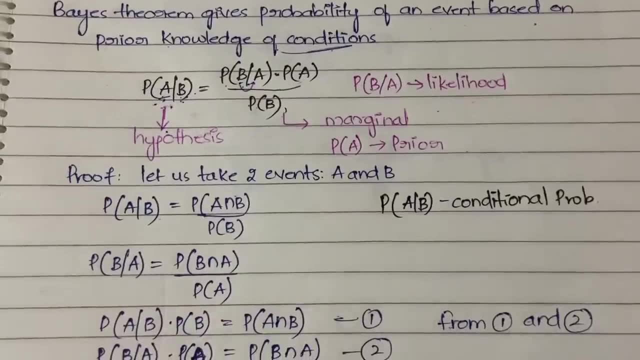 P of A by B as Okay Done. So now let us see the proof of this formula, and then let's move over to the next. Right Now, according to the conditional probability, we know that P of A by B is equal to P of. 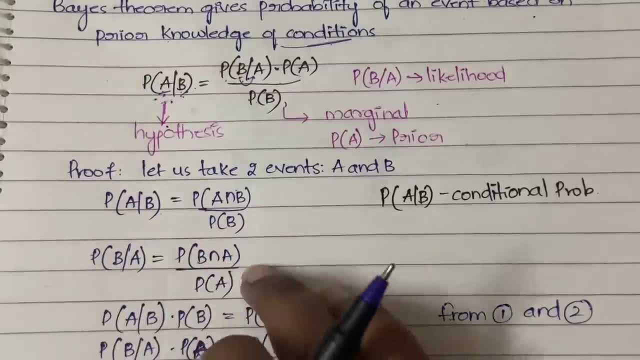 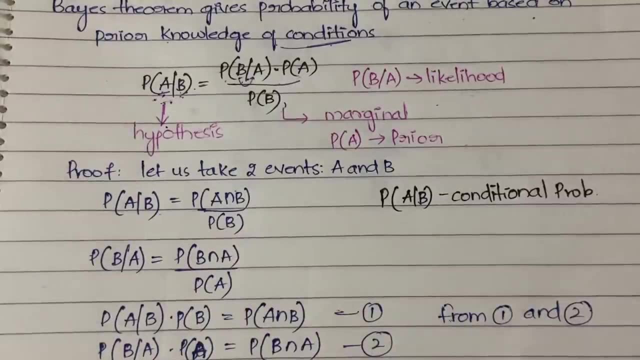 A intersection B by P of B Right, And P of B by A is equal to P of B, intersection by P of B, intersection A by P of A. So these two are the formulas for conditional probability. Now again, don't confuse. from where did we get this? 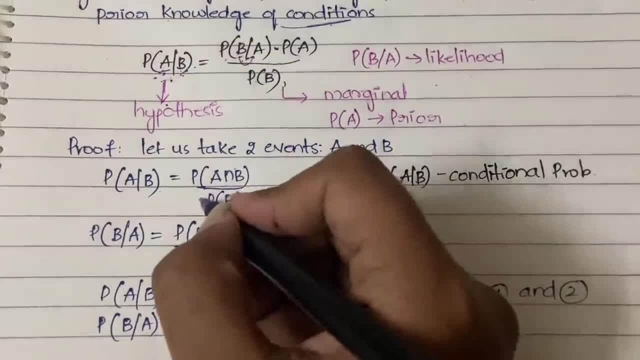 Okay, Right, So now what do you do? You send this P of B over to this side and P of A over to this side. Okay, So you send this P of A over to this side, and what do you get? 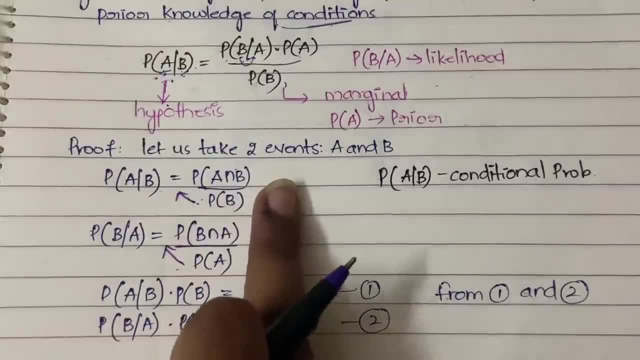 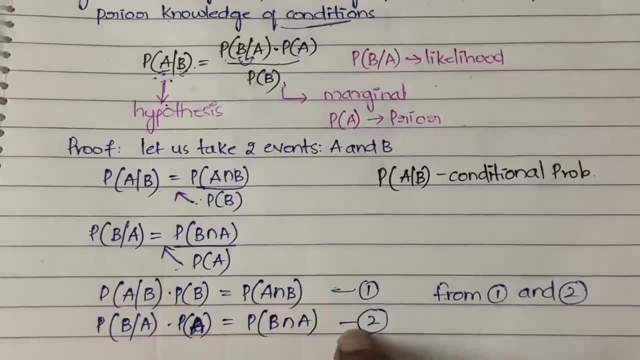 P of A by B into P of B is equal to P of A, intersection B, Right? So that is what we got here And here also sending P of A to this side. P of B by A into P of A is equal to P of B intersection. 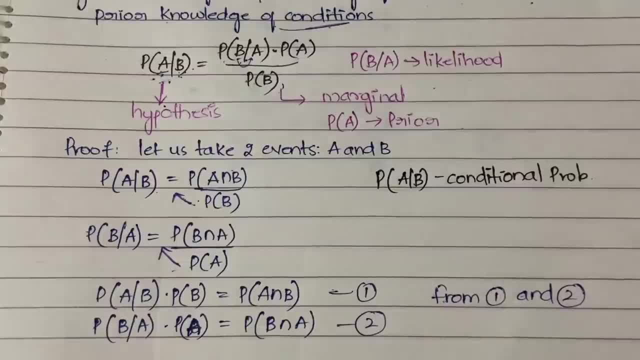 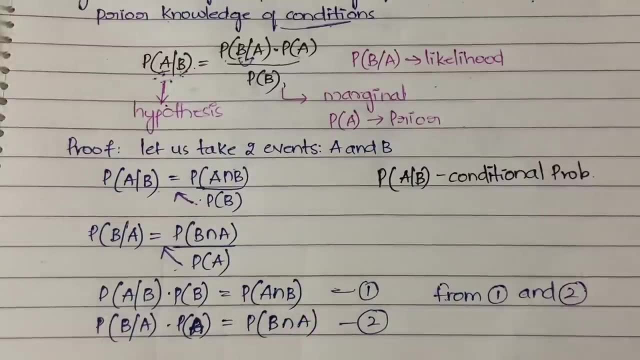 So that is the second equation. So we got two equations And you see, here we have A intersection B and here we have B intersection A. A intersection B means what Common in both A and B, Right And B intersection A means what? 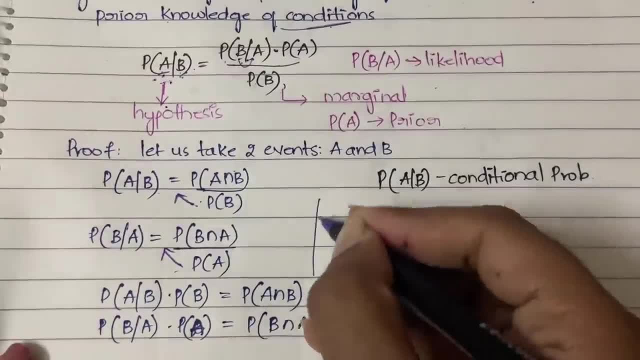 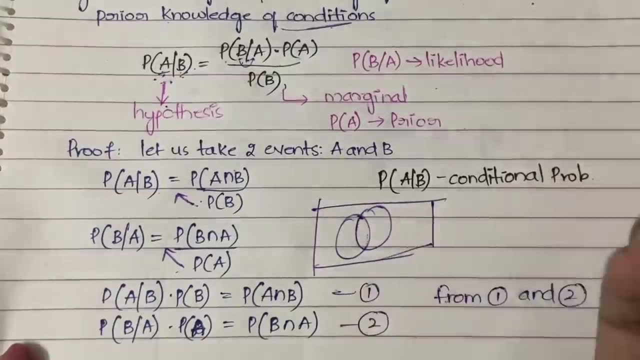 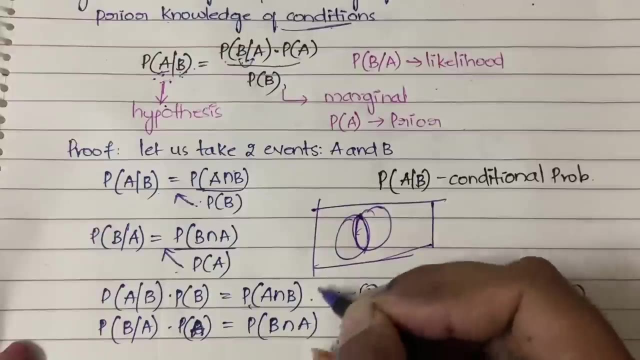 Common in both A and B, again Right, when diagram has. so this is a and this is b. so a intersection b means this part right and b intersection a, also this part only. so both of them means the same. so p of a intersection b and p of b intersection a, both are equal actually. so when these two are equal, when the rhs part is: 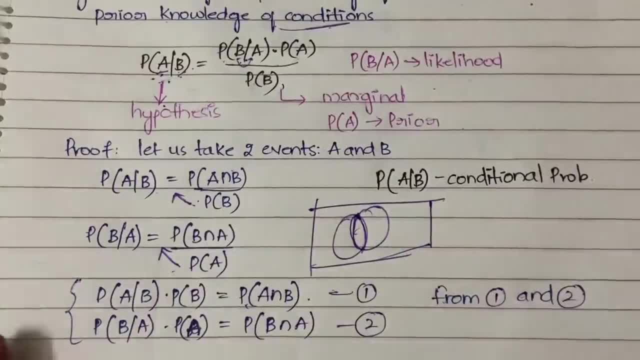 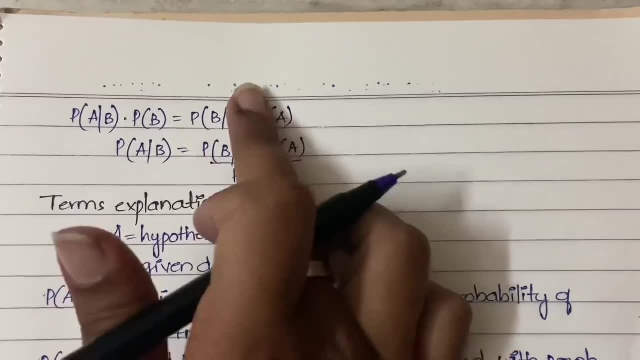 equal. you can obviously equate these two as well, right? so let us see what you get when you equate on equating both of them. you get: p of a by b into p of b is equal to p of b by a into p of a. okay, 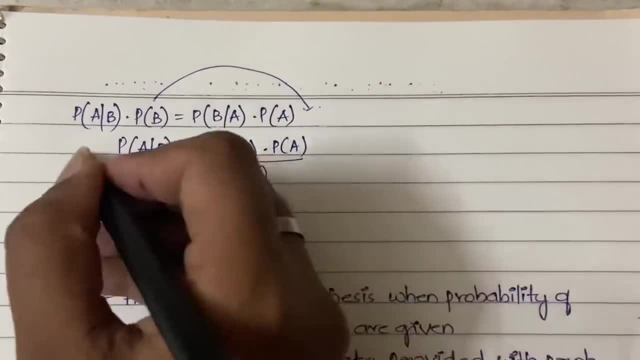 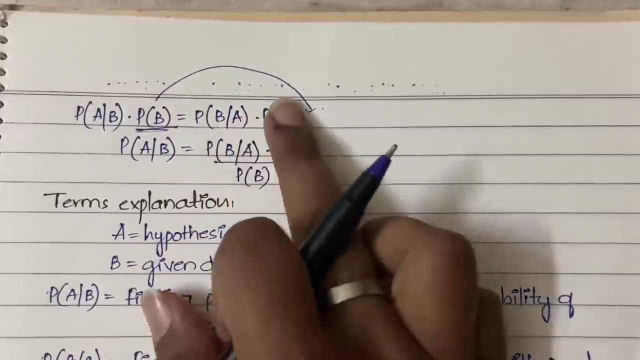 now what you have to do is send this p of b over to this side. here it is a numerator. right on coming over to this side it comes to the denominator, so p of a by b will become p of b by a into p of a by. 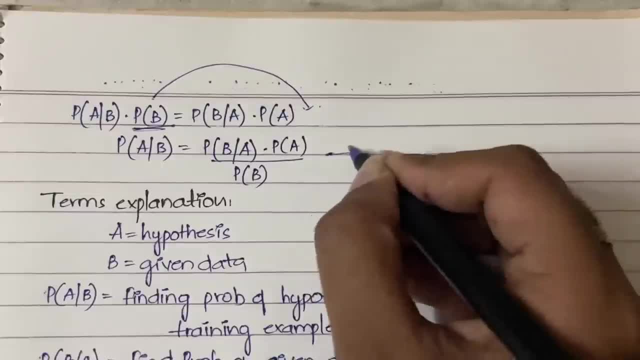 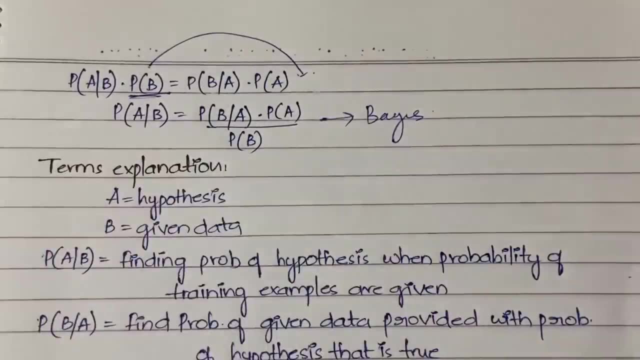 p of b. okay, done so. this is what. this is nothing but our base theorem, right? so now i will explain you the terms: weight. so a is called as the hypothesis and b is called as the given data, not called actually. so a refers to the hypothesis and b refers to the given data. right from the given data we have. 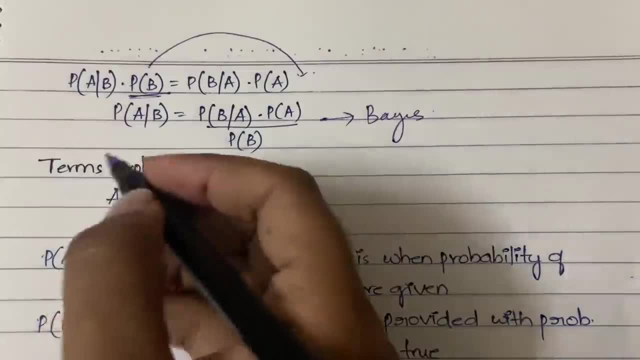 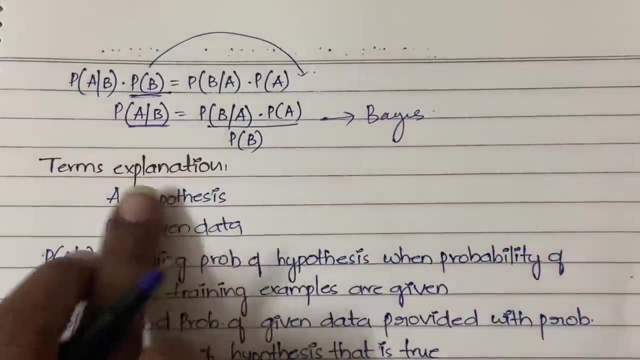 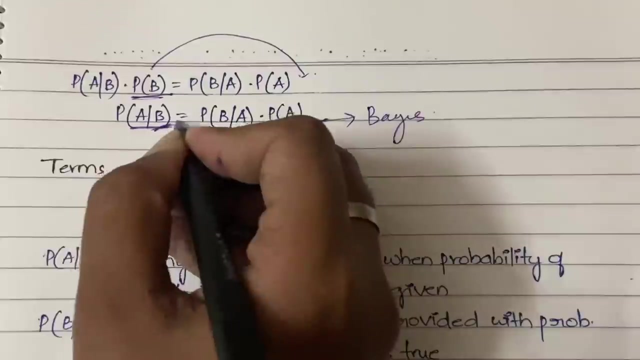 you know, figured out a hypothesis and that hypothesis is represented by a and b stands for the entire given data. now, what is a of a by b? you need to find the probability of hypothesis. that is a when the probability of training examples are given. okay, so b has already occurred, right a? 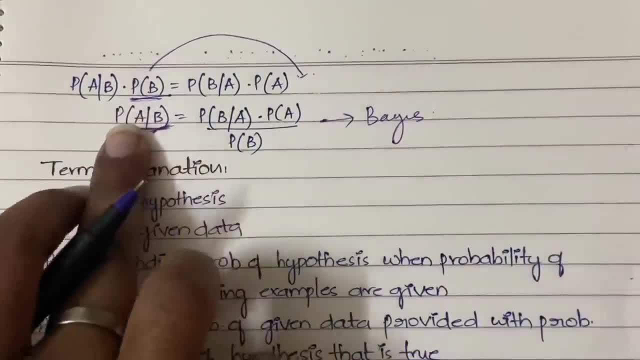 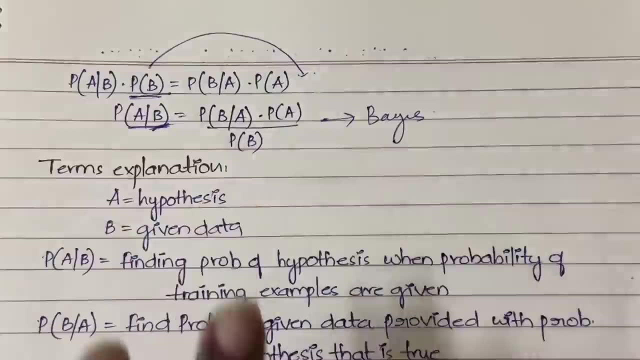 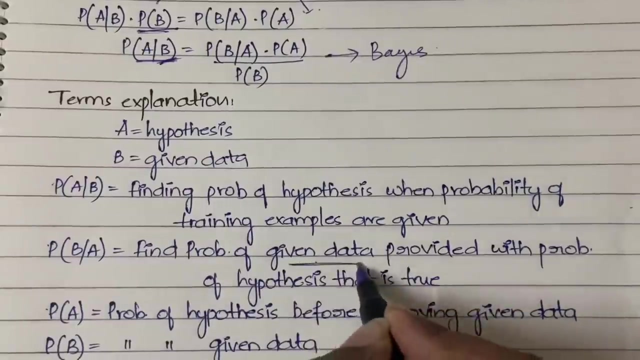 by b means so: yeah, so you need to find out the probability of a, given that the probability of b is given to you. okay, so that is p of a by b. next is p of b by a. so how do you find out the probability? sorry, what is p of b by a? finding the probability of given data, provided with the probability of. 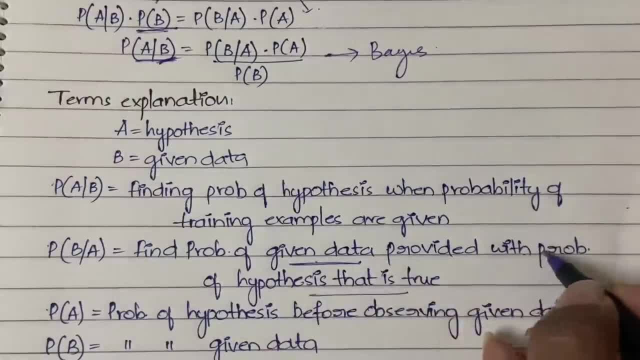 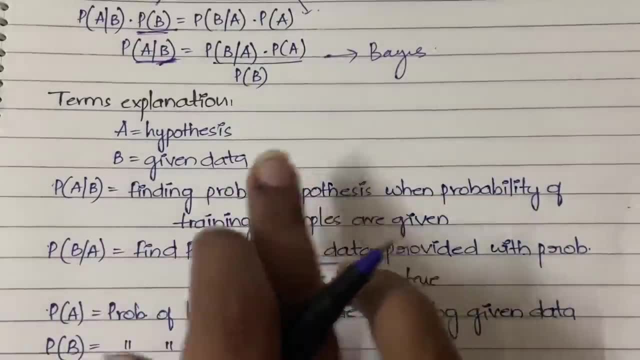 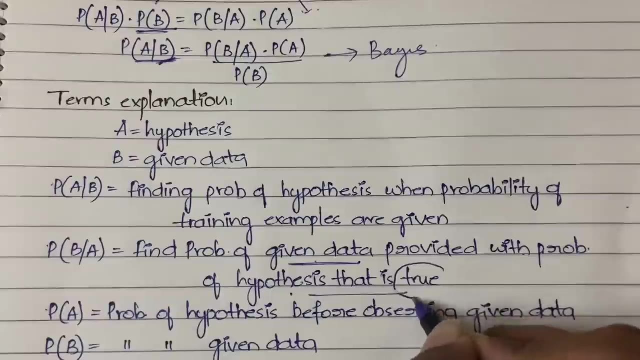 hypothesis. that is true. you are provided with the hyper probability of hypothesis here and you need to find out the probability of given data. here you need to find out the hypothesis, the probability of hypothesis, when the given data's probability is given. try to understand the difference, and here you're going to take the probability of hypothesis only. that is true of the hypothesis. 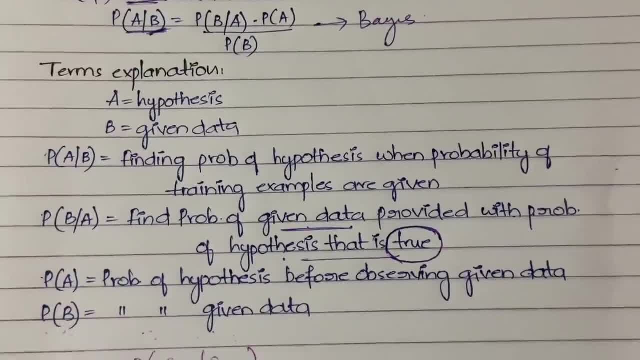 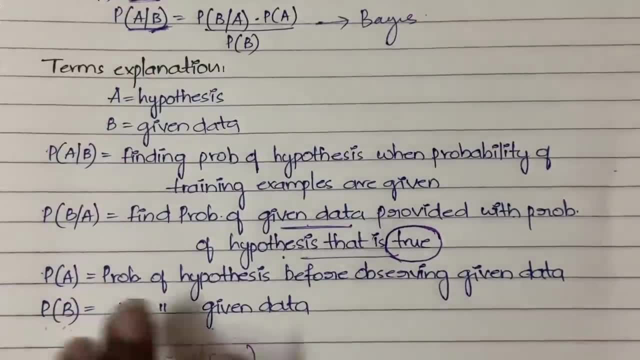 that is true right now. next is p of a. so what do you mean by p of a here? the probability of hypothesis before considering the given data, right, and what is p of b? probability of given data. that's all so simple explanation of all the terms done, and i already explained so what. 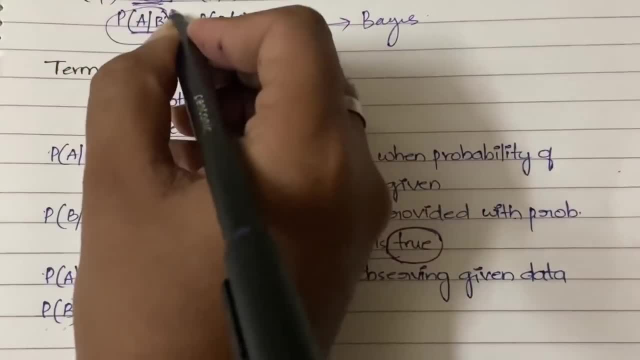 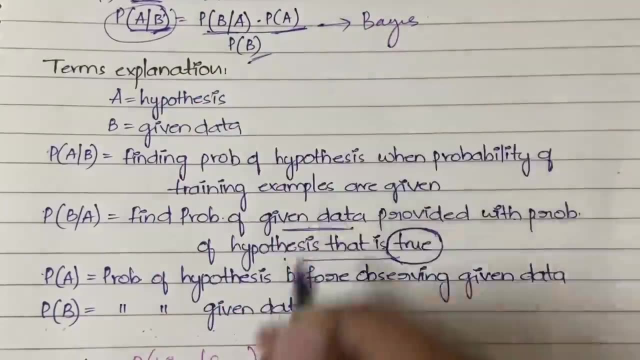 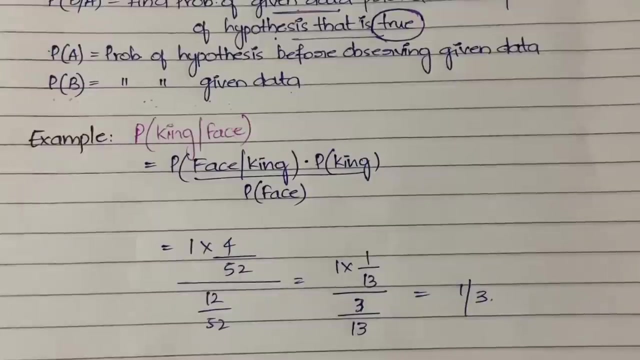 are the terms means. so here this a by b is hypothesis and this b by a is called as the likelihood, p of a is called as the prior and p of b is called as the marginal. okay, done now. so we are done with the terms explanation. now let us try to understand an example and 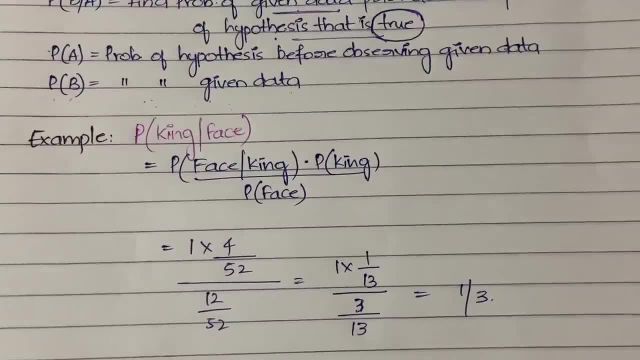 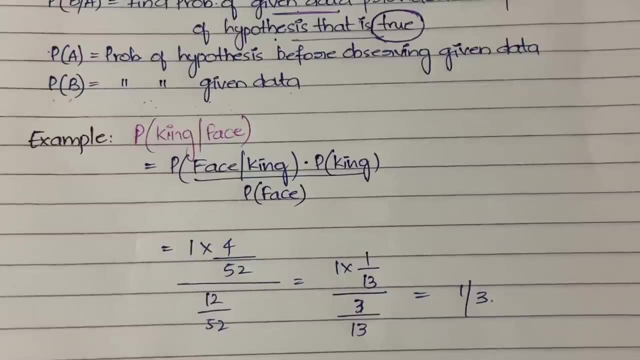 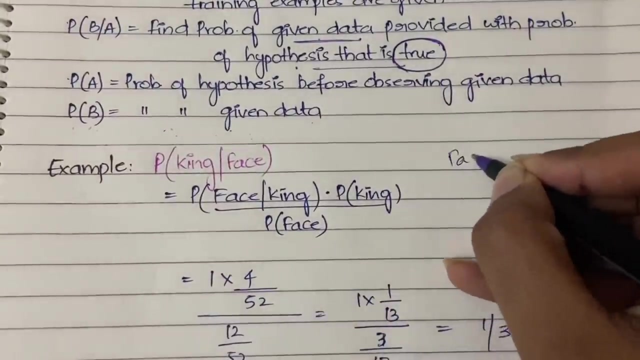 let us close that. so p of king by face. so you know cards, right, we play cards. so in that, p of king by face. so what is? what is the meaning of that probability of finding a king, given that it is a face card, right? so yeah, how many face? what do you mean by face cards? actually, face cards means j k q, right? 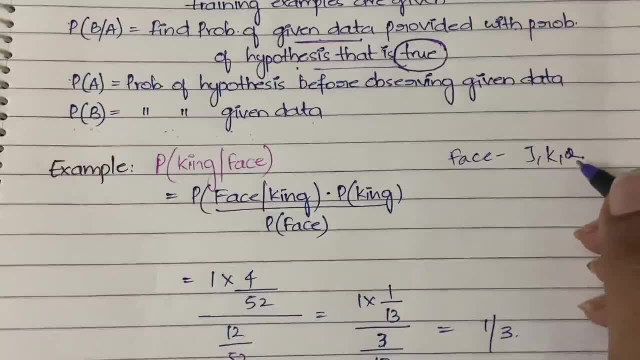 so these three are called as the face cards. so how many face cards you have? so for each set, we have for diamond, we have a spade, we have for heart, we have like that. for each set we have three right total we have four sets. four into three you'll have total of. 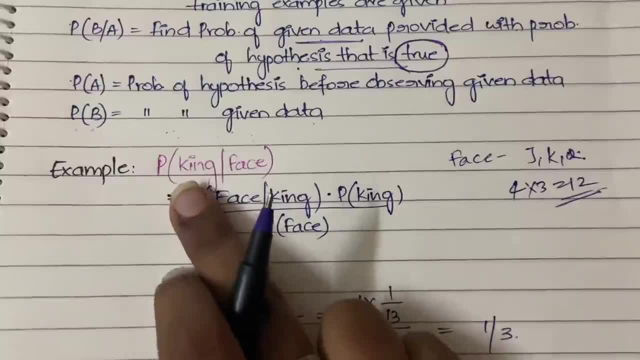 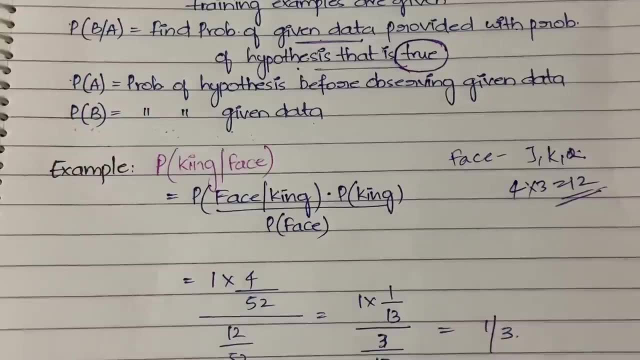 twelve face cards, right? and so how do you elaborate this formula, face by king, into probability of king by probability of face? so what do you mean by probability of face by king? pro, you need to find out the probability of a face card, given that it is a king. obviously all kings are face cards, right? you take diamond, or you take spade, or 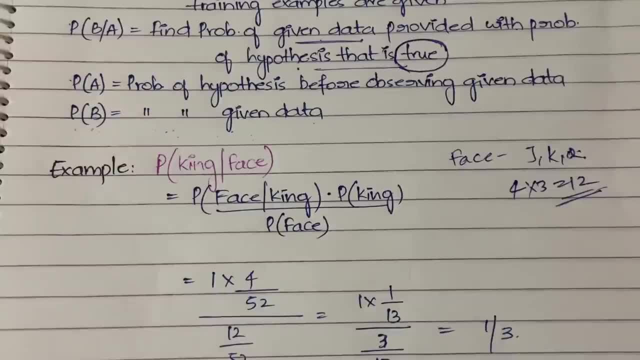 you take heart or you take the other one. all of them, it is face card only, every king is a face card, so obviously the probability would be one. so how many face kings you have? three, sorry, four, four right total, and how many kings you have four. so four by four you'll have: 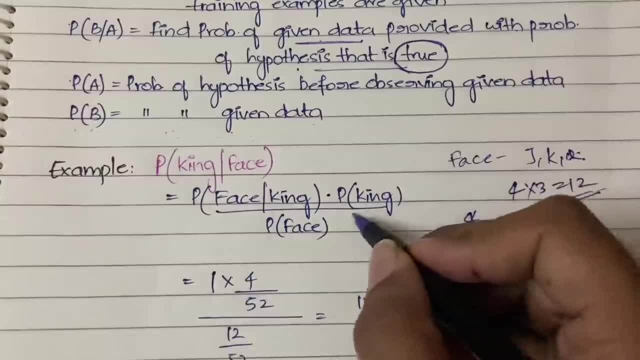 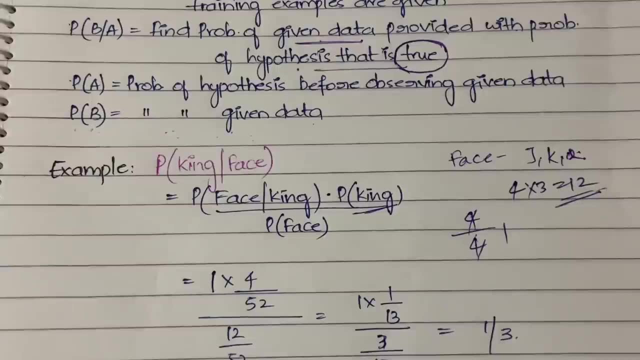 four, you'll get one as a probability. so one into p of king. so probability of king among fifty two cards. how many kings you have in fifty two cards? you have four kings right. so for heart one, for the spade one and for diamond one, and for the other one i am not. 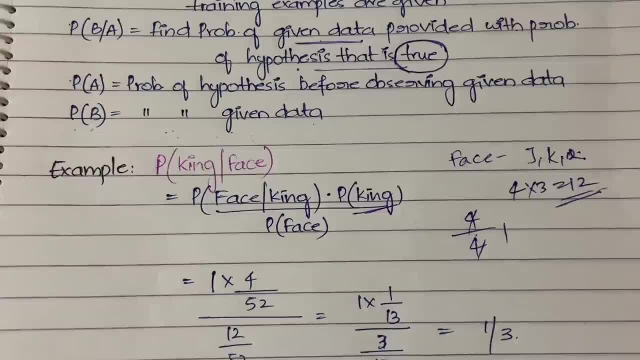 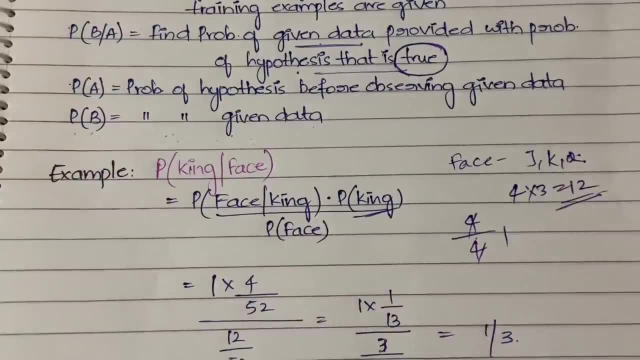 getting its name. so for the other one you have one. so total four kings you'll have. so four by total of fifty two cards. four by fifty two by probability of face. probability of face in the sense: number of face cards by total number of cards, right? so how many face? 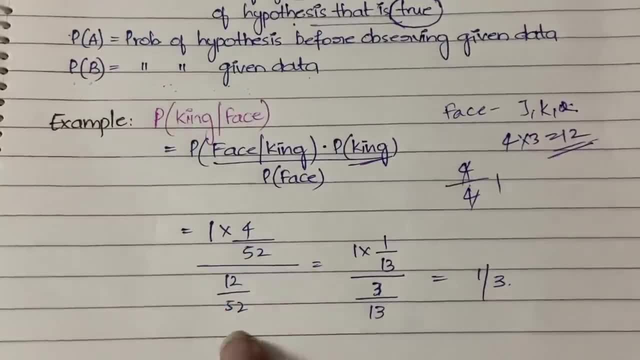 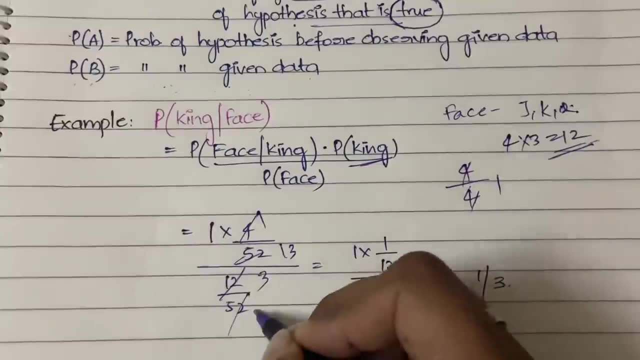 cards you have. so twelve by total number of cards you have is fifty two, right? so when you cancel, four ones are four, four thirteens are fifty two and four. threes are twelve and four thirteens are fifty two. yeah same, so you'll get one by thirteen, by three by thirteen. 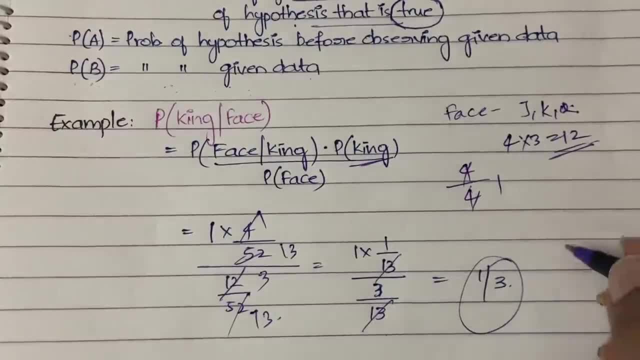 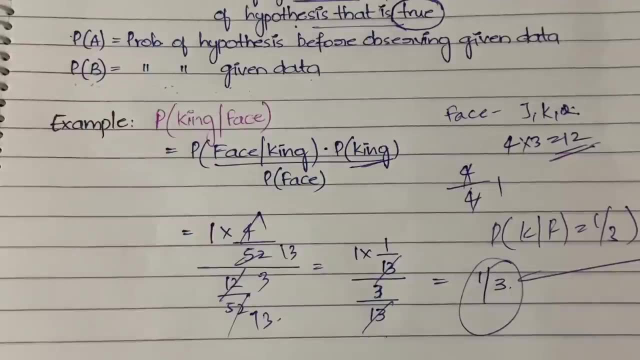 thirteen, thirteen, cancel. you'll get one by three as the probability. so what is probability of king by face? it is one by three. ok, done so. this is how you need to do. you need to apply the base theorem. ok, done So for how many kings you have? you need to apply the base theorem. ok, done so for how. 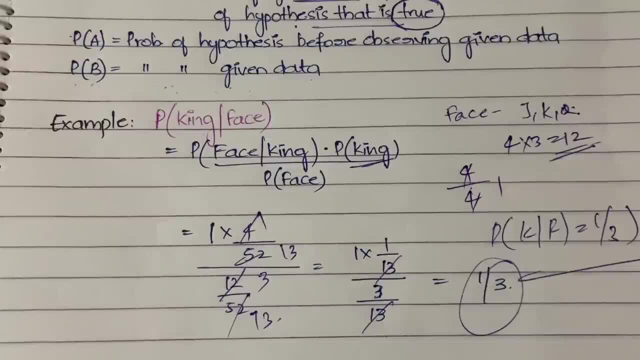 what, in which situation, base theorem is useful for you? it will give you the probability of an event based on the prior knowledge of the conditions. be based on the previous knowledge of the conditions. you're going to get the probability ok, done so. this is about the base.